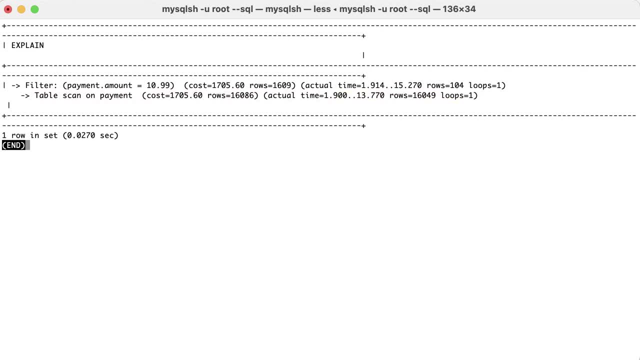 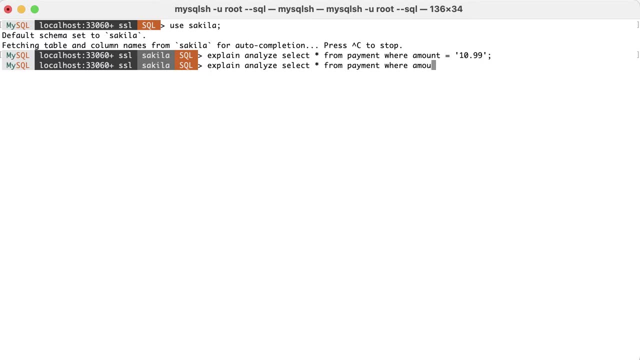 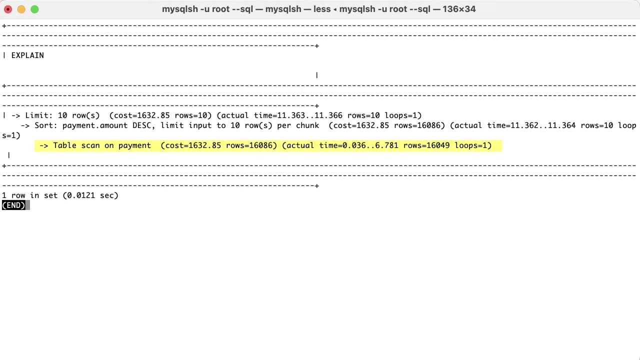 Since there is no index, MySQL will use a table scan. We want to return the 10 most expensive payments from the table. Again, MySQL will do a table scan and then, with the results, process a sort operation which takes 11 milliseconds. 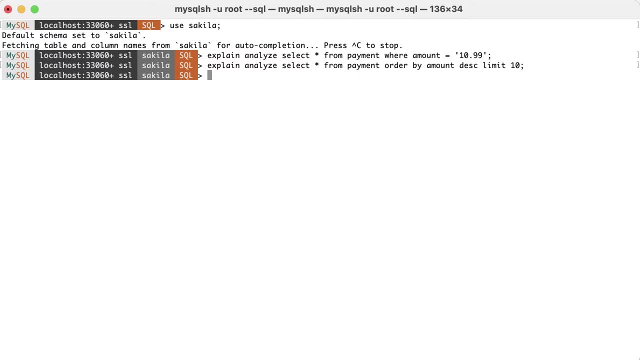 If the queries above are executed frequently, then it would make sense to add an index. ALTER TABLE PAINTMENT. Add index for the amount column. This time, if we execute the first query again, we can see that the index is applied and also. 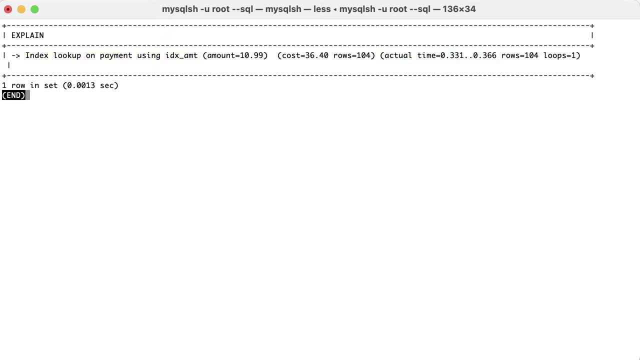 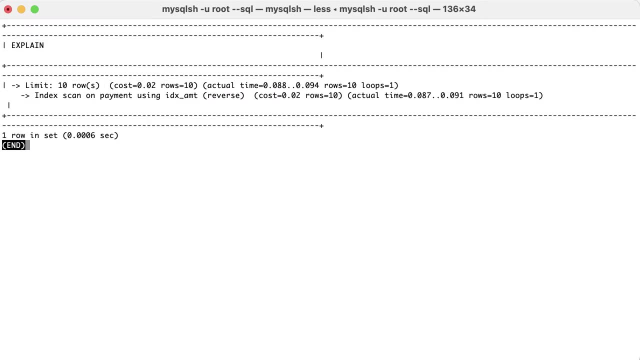 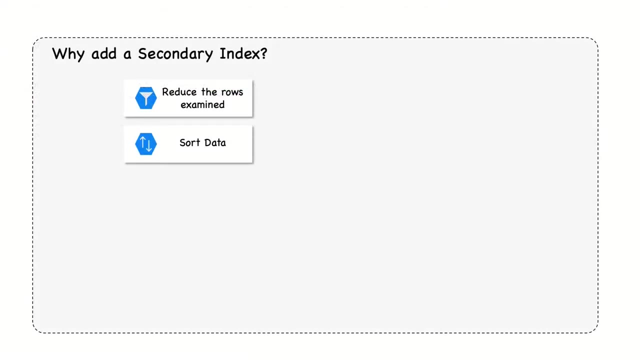 the execution time is smaller. Similarly, if we execute the second query again, we'll see that MySQL will just read the index to retrieve the rows in descending order. There are also some other use cases for indexes. We can validate data. in this case, we can benefit from the indexes that are unique. 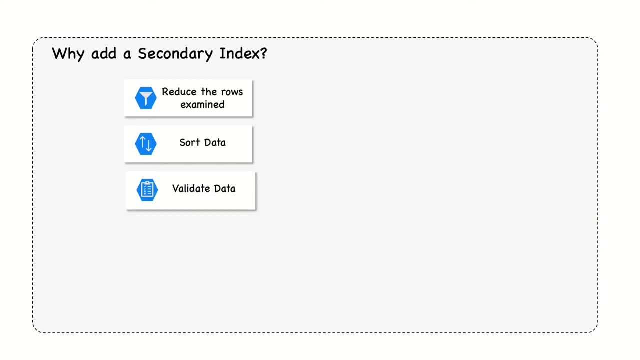 to allow only distinct values for a certain column. Also, we can use the index to avoid eroding the rows from the table, since for covering indexes, we can return all the required data without reading the whole row. Finally, we can use the index to find minimum and maximum values. 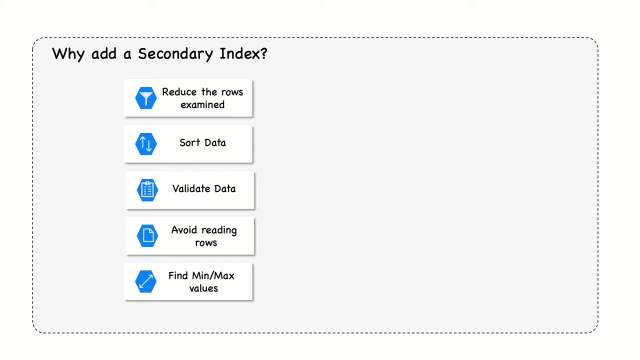 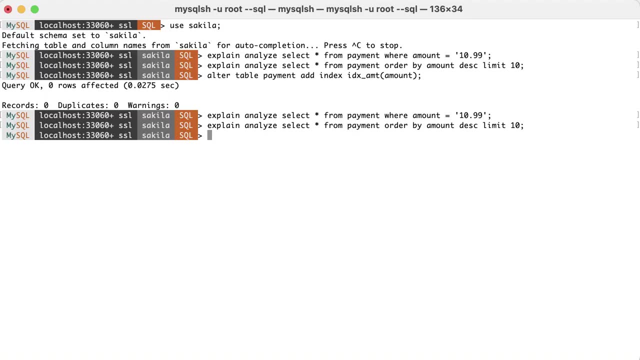 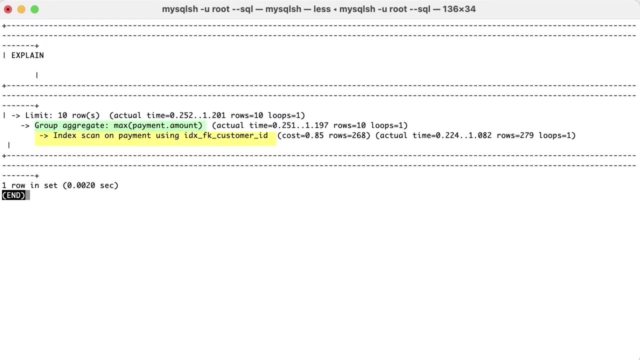 For group by values. the minimum and maximum values for an index column can be found by just checking the first and last records in the index. For example, select Customer ID, Max Amount from Page Rate, Month. Group by ID and Limit to 10.. 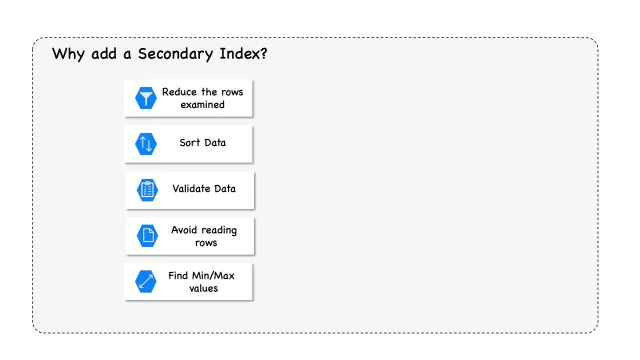 When you need to decide whether to add an index, you need to ask yourself which of these purposes the index is needed for and whether it will be able to fulfill them. Don't take the work of adding an index lightly, as the difference in response time between 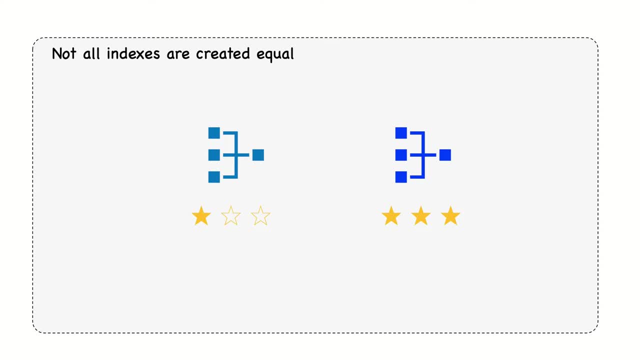 great and poor indexes can be several orders of magnitude. Index maintenance is a never-ending task. It starts when we first add the index to the table and continues throughout the lifetime of the table. Indexes may affect not only the raw query performance but also locking memory and 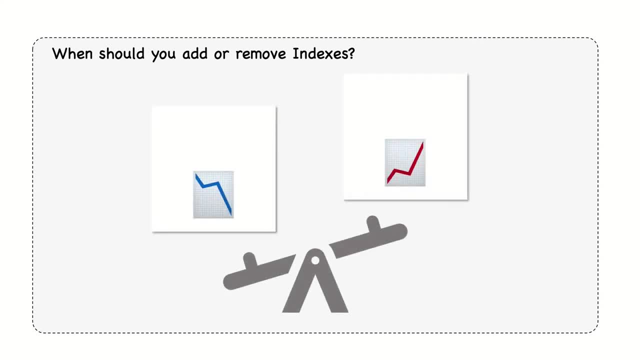 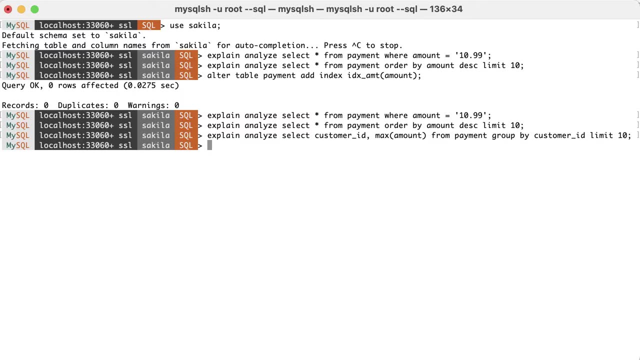 CPU. So to justify the existence of an index, we should use statistics to determine its usefulness and efficiency. There are two main views in the SIS schema that can help to find statistics with full table scans. We have schema tables with full table scans. 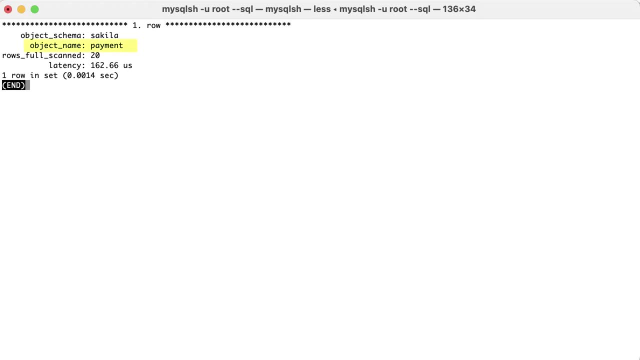 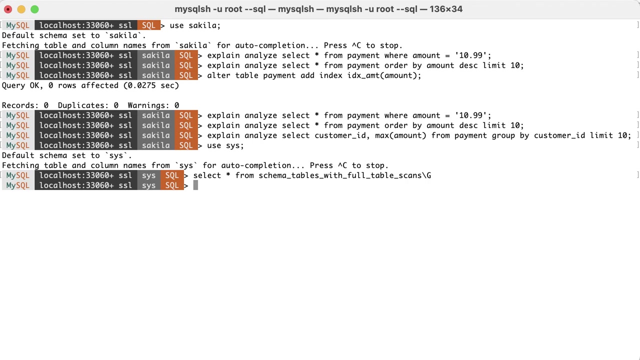 This view shows all tables where rows are read without an index. The output is sorted in descending order by the number of rows. If a table has a large number of rows read, you can look for queries using this table and see if indexes can help. 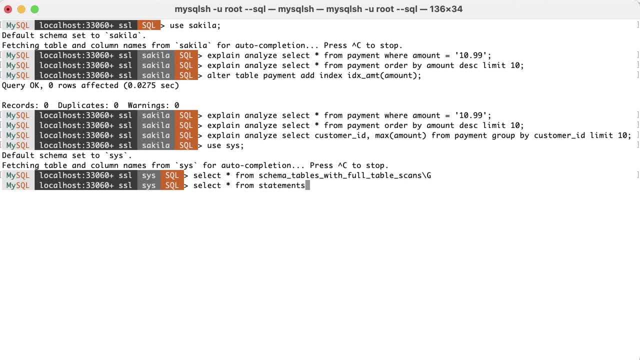 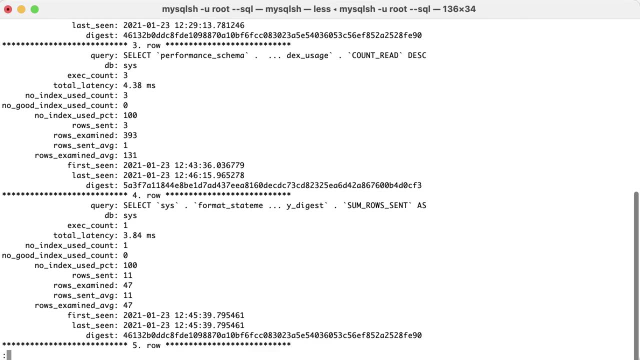 Then we can use statements with full table scans. This view shows the normalized version of the statements that don't use an index at all or don't use a good index. The statements that don't use a good index are the ones that don't use a good index. 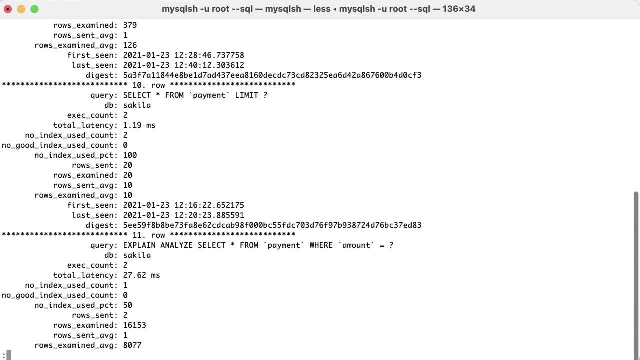 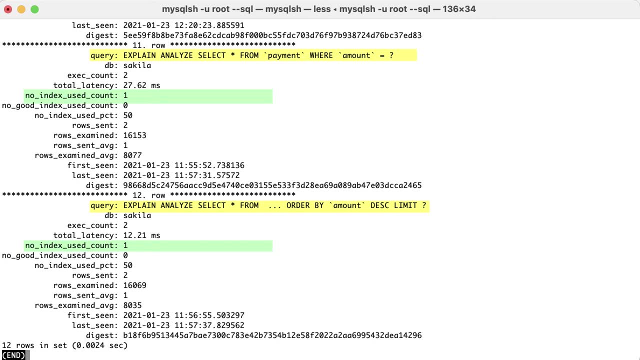 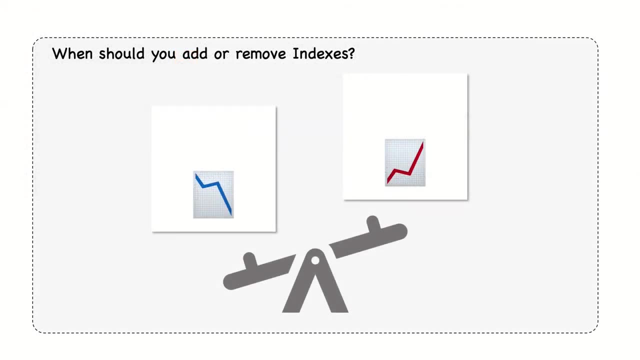 The statements are ordered by the number of times they have been executed without using an index at all and then by the number of times they haven't been using a good index, both in descending order. When you identify that queries can benefit from additional indexes, then you need to. 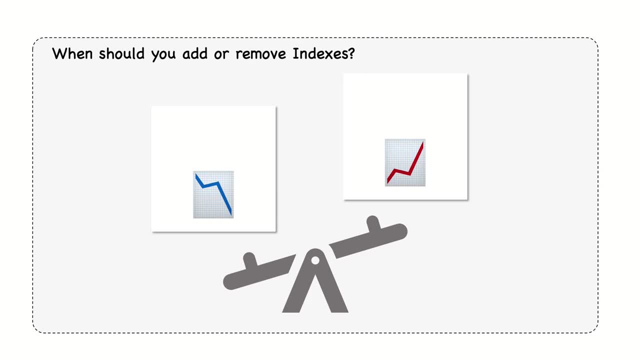 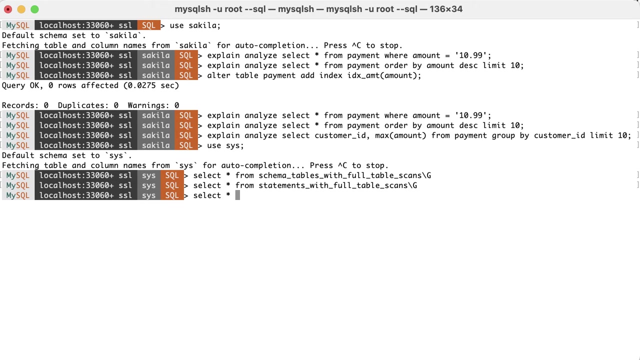 evaluate whether the cost of having an extra benefit is worth the gain when executing the query. Therefore, in addition to these views, we also need to keep an eye on the performance of the query. The performance schema and the sys schema are particularly useful to find indexes that are 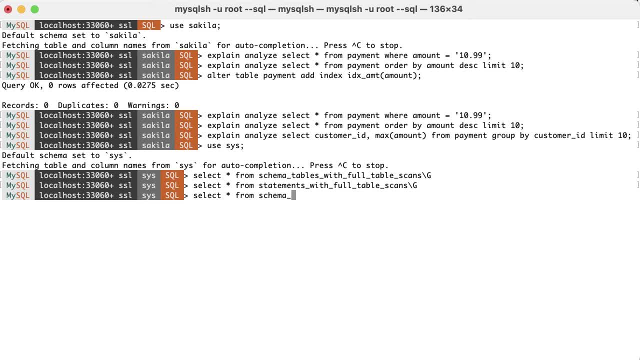 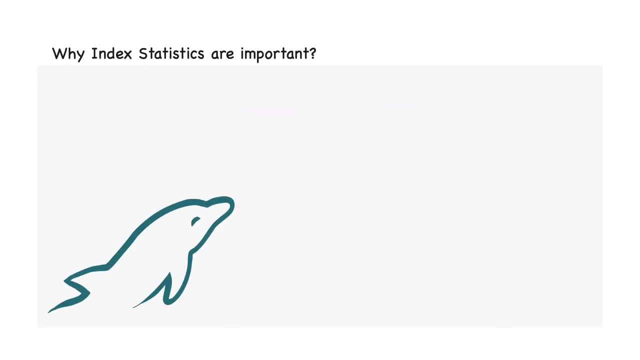 not used anymore or not used at all. First, we have schema unused indexes, And it can also be useful to check schema redundant indexes. When MySQL decides whether to use an index or not, it boils down to how effective MySQL thinks the index is for the query. 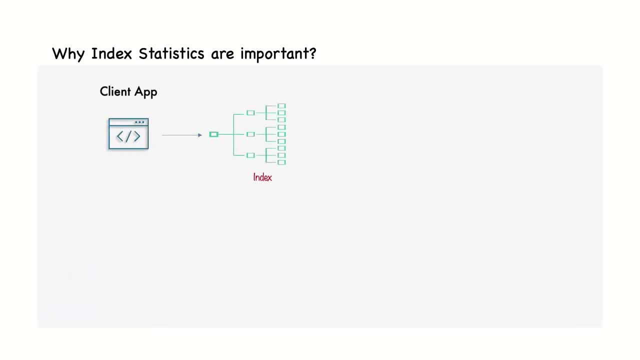 Remember that when we use a secondary index, there will be an extra primary key lookup to get to the data. Also, secondary indexes are not ordered in the same way as the rows, so using the index will mean, in general, a random IO. 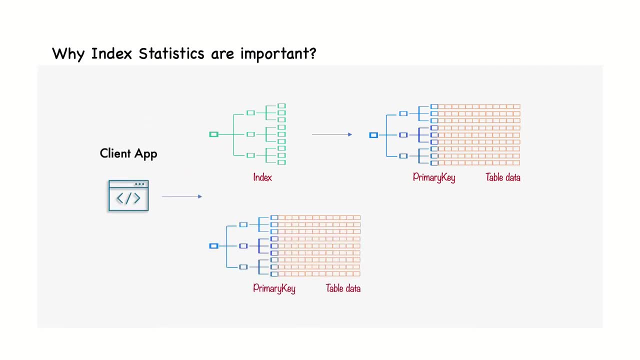 A table scan, on the other hand, is, to a larger degree, sequential IO. So row for row doing a table scan is cheaper than finding the same row using a secondary index. This means that for an index to be effective, it must filter out a large part of the table. 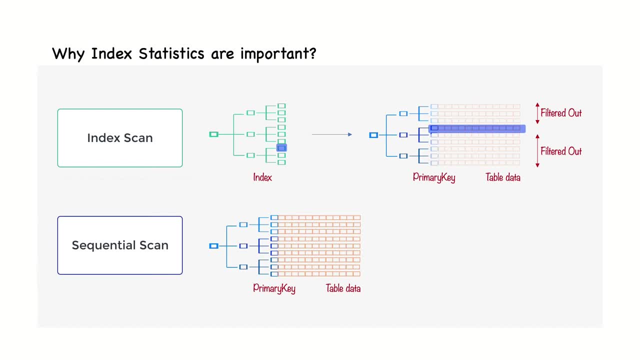 Exactly how much must be filtered out depends on the performance characteristics of your hardware. how much of the table is in the buffer pool, the table definition and more. In the days of the old spinning disks, the rule of thumb used to be that if more than 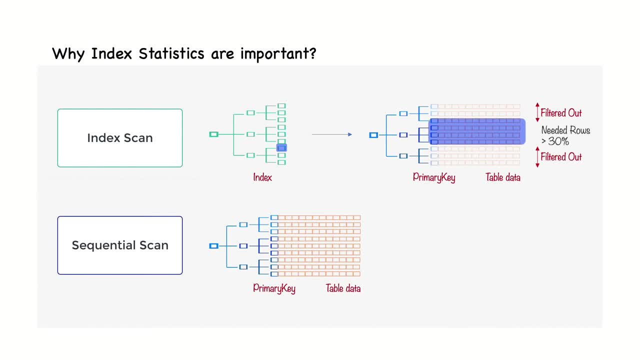 30% of the rows were needed, then a table scan is preferred. So normally, the more of the rows that are in memory and the better the random IO performance of your disks, the higher this threshold will be. This is where index statistics come into picture. 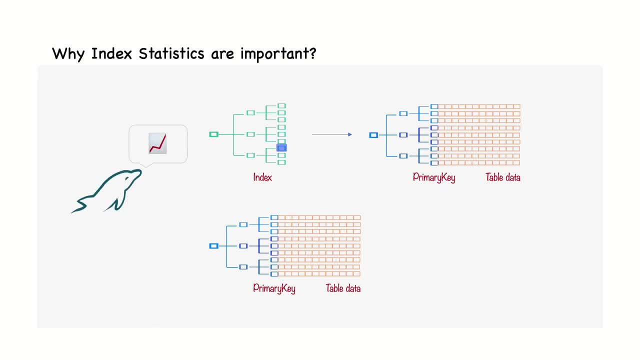 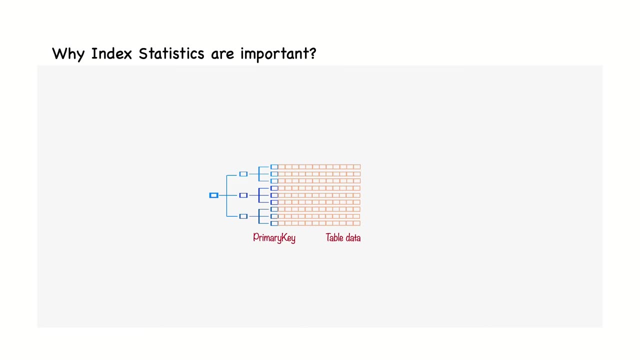 The optimizer, which is the part of MySQL that decides which query plan to use, needs some simple way to determine how good an index is for the given query plan. The optimizer obviously knows which columns the index includes, but additionally it needs some measure of how well the index filters the rows. 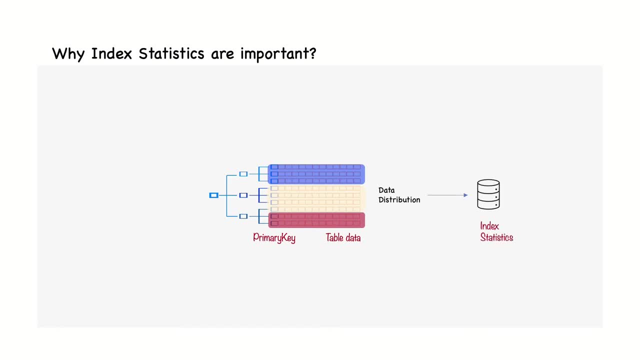 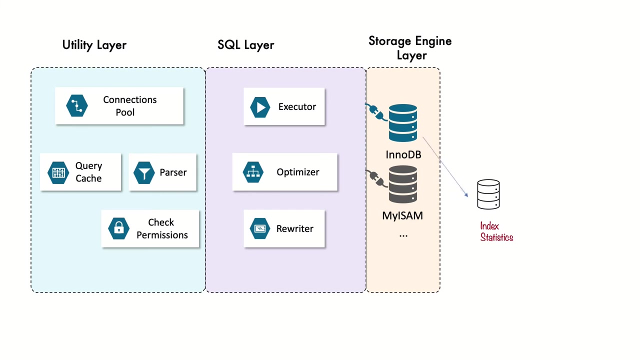 These kind of facts are found in index statistics, which provides approximate information about the distribution of data in an index. In MySQL, it is the storage engine that is responsible for providing the index, So it is worth looking more into how InnoDB handles index statistics. 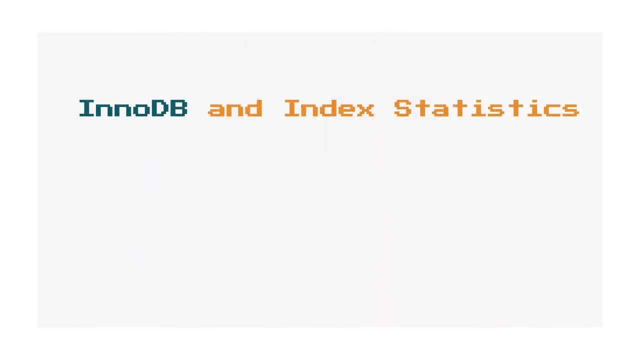 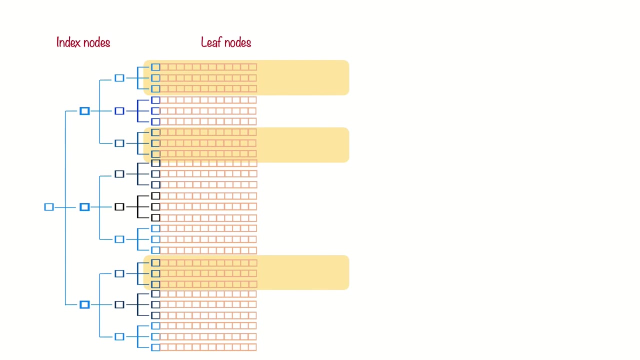 InnoDB calculates its index statistics by analyzing random leaf pages of the index. It may be, for example, that 20 random index pages are sampled, which is also called 20 index dives, And it is examined which index values those pages have. 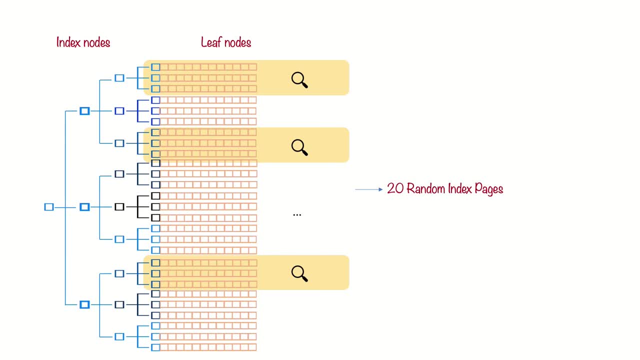 Then InnoDB scales this based on the total size of the index. An important implication of this is that InnoDB index statistics are not exact. Why are estimates used instead of exact statistics? The reason is performance. Calculating the index statistics has an adverse effect on query performance. 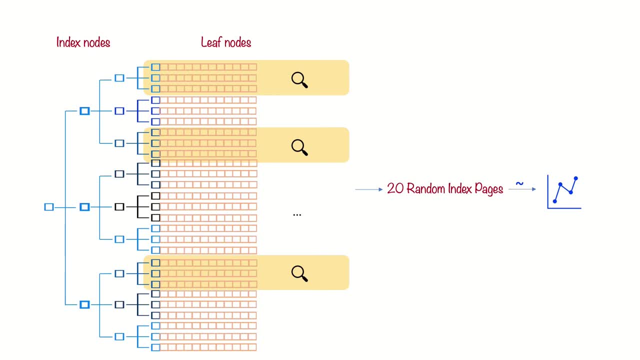 So it has been chosen to limit the scans to a relatively small number of pages. The downside of using approximate statistics is that they are not always a good representation of the actual distribution of values. When this happens, the optimizer may choose the wrong index or the wrong join order, causing 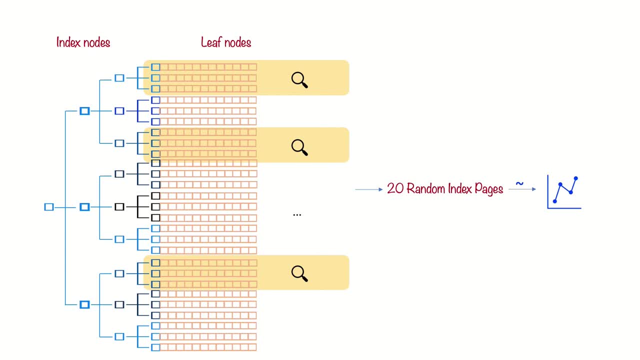 slower queries than necessary. However, it is also possible to adjust the number of random index dives. How to do this depends on whether persistent or transient statistics are used. In InnoDB, the index is set to the value of the index. In InnoDB, the index is set to the value of the index. 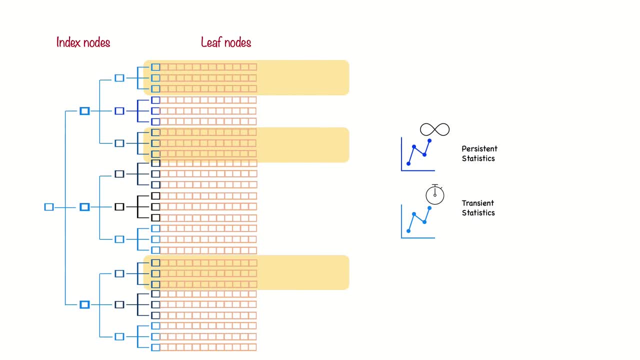 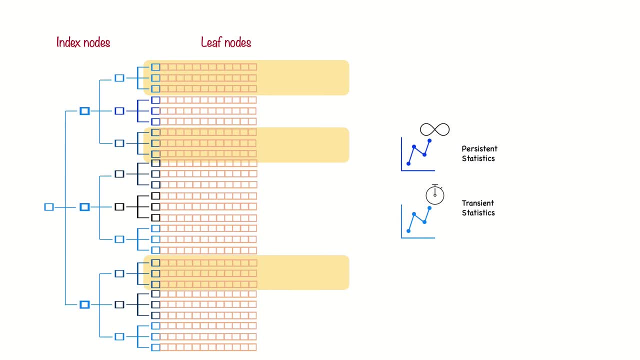 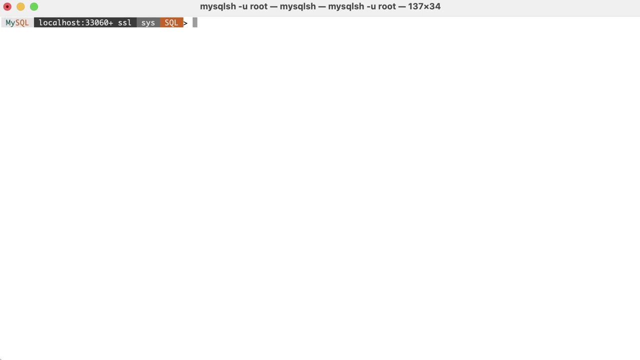 allow to sample more pages, they are updated in the background and they can be configured to a larger degree, including support for table-level options. Persistent statistics: use this option as the default number of pages to sample. Persistent statistics: use this option as the default number of pages to sample. 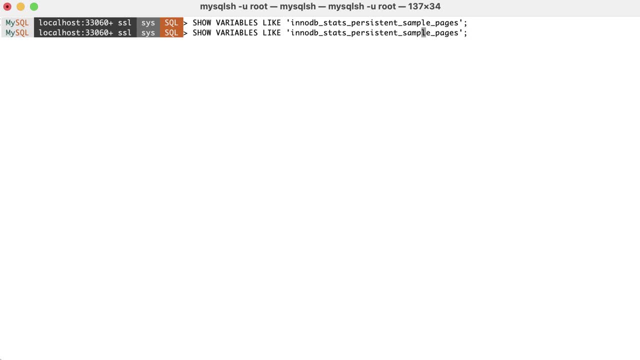 And transient statistics use the number of pages specified by this option. However, these too are global variables. To override this kind of system-wide settings, it is recommended to configure them for individual tables. Therefore, we can define stats in Create Table or Alter table gum. 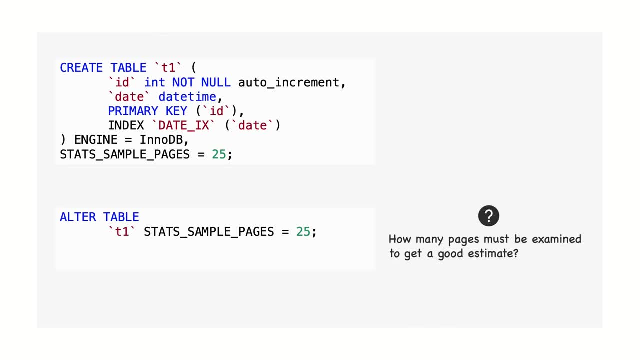 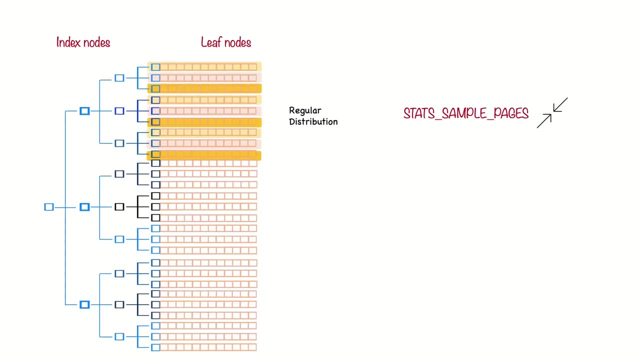 Therefore, we can define stats in Create Table or Alter table. gum table statements. But how many pages must be examined to get a good estimate? That depends on the table. If the data distribution is uniform, that is roughly the same number of rows per index.